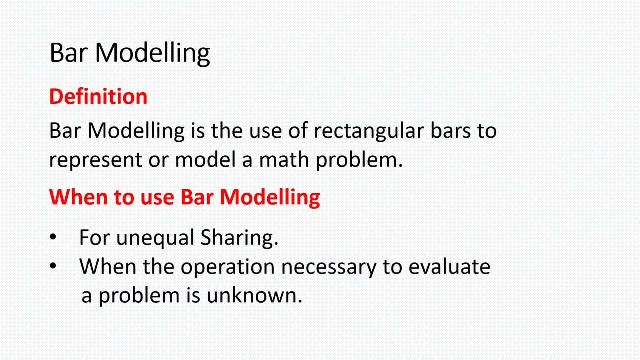 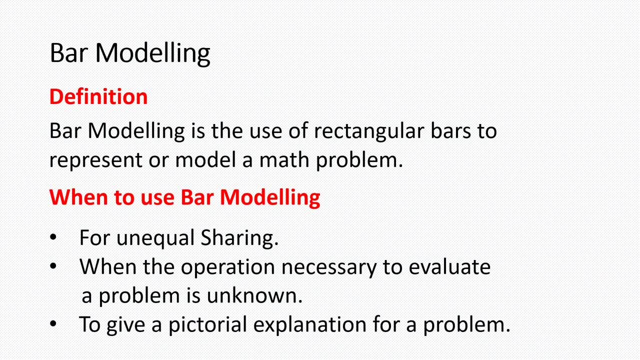 The first of which is for only point sharing, The second of which is when the operations necessary to evaluate a problem is unknown. The third situation in which I would recommend the use of bar modeling is to give a pictorial explanation for a problem. Here's a good example: 360 people. 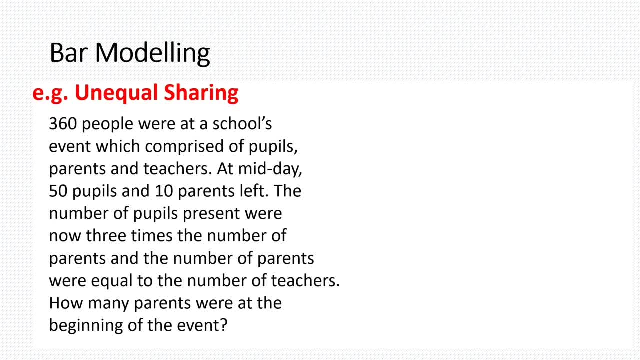 were at a school's event which comprised of pupils, parents and teachers. At midday, 50 pupils and 10 parents left. The number of pupils present will now three times the number of parents and the number equal to the number of teachers. How many parents were at the beginning of the event? 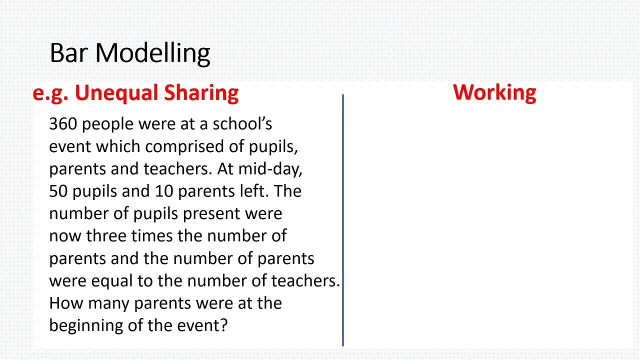 Here's my working column To evaluate this. as mentioned before, we are going to use bar modeling. This bar will therefore represent the 360 people that were initially at the school event. Recall that 50 pupils left and 10 pupils left In bar modeling. remember we emphasized on spatial 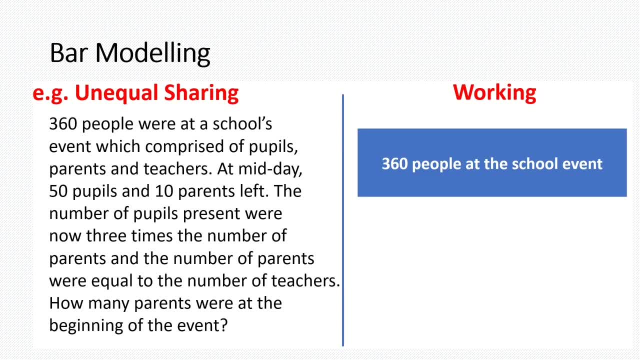 equality or spatial equality. This bar represents the number of pupils that were initially at the event, So that if I were to represent 50 pupils and 10 parents, then the bar that represents the pupil must be bigger than that of the bar representing parents, Like this. 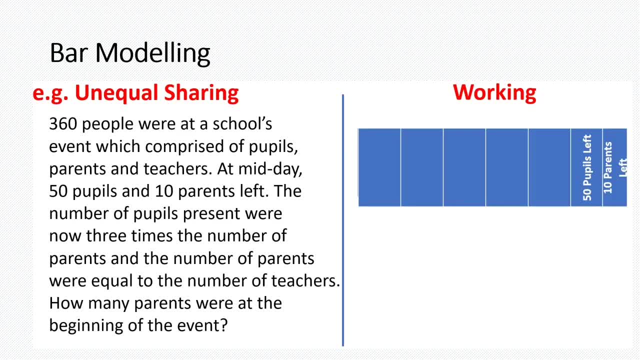 Recall also that after the pupils and the parents left, the number of pupils present was three times the number of parents, and the number of parents was equal to the number of teachers. This means that the number of pupils that were initially at the event would be divided into five equal parts. 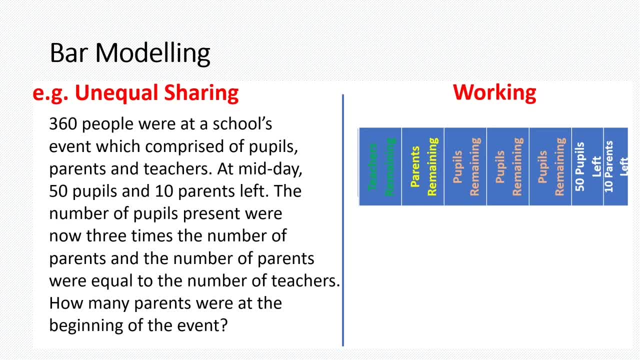 This, therefore, would be a better representation of the problem. Here you can see 10 parents left, 50 pupils left, and we will have three times the number of pupils as parents, and the bar representing parents will be equal to the bar representing teachers, So that the entire bar will. 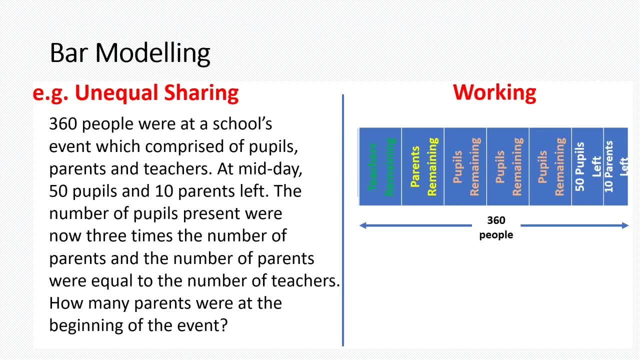 be equivalent to 308.. people. but to proceed with the problem, we need to take out those that left, so we will have 360 minus 50 minus 10, which will give me 300 people remaining. the 300 people remaining would be these bars. recall that each of these bars equals each other. 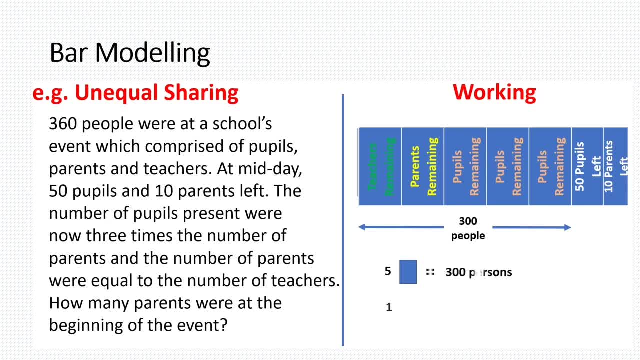 so, therefore, five of these bars will be equivalent to 300 persons, and so, therefore, one of the bars will be equivalent to 300 divided by 5, which is equivalent to 60 persons. this means that each of the bars that are of equivalent width and area would be equal to 60. 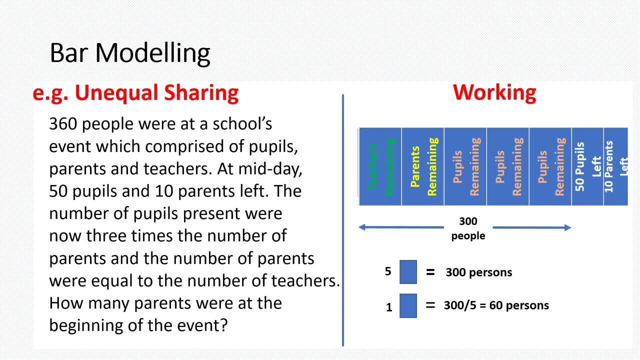 persons, but recall the question asked how many parents would be present at the beginning of the event. recall that 10 parents left at midday. so to get all the parents that were at the beginning we need to add 60 to the 10, which would give me 70. so at the 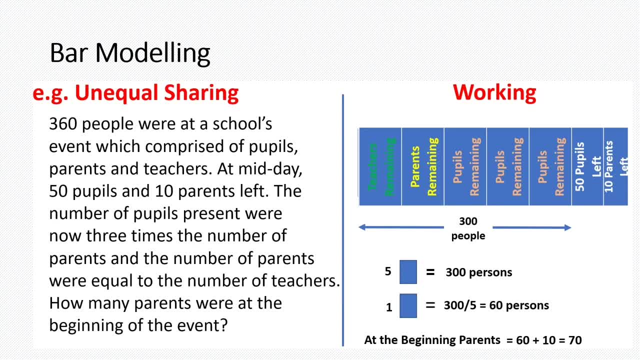 beginning of the event there was 70 parents present. this also illustrates an important point that we made earlier. immediately, we could not have immediately deciphered the operation necessarily to evaluate the problem. bar modeling helps you to visualize the problem and therefore helps you to choose the correct operation to evaluate the problem. so therefore, 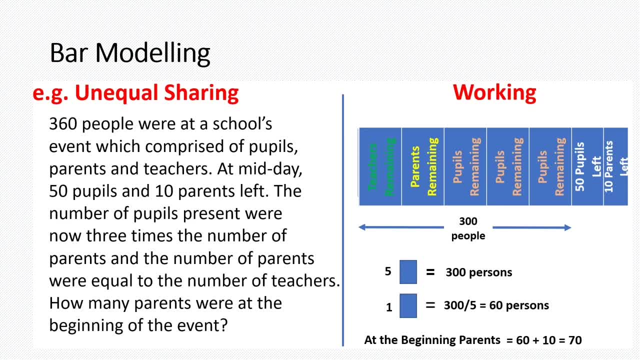 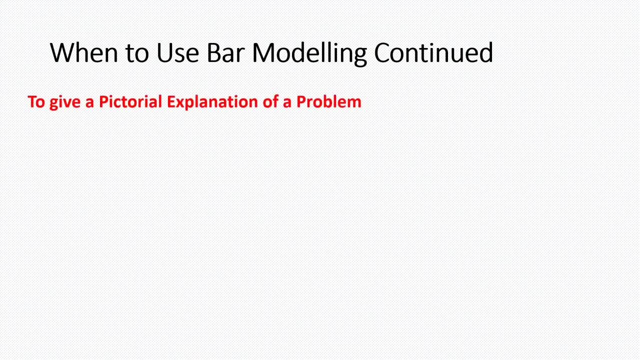 let's look at the last situation, which you can use bar modeling for the seo examination. the final advice when to use bar modeling was when you are given a problem and you are required to give an explanation for your answer. this can be done pictorially. here is an. 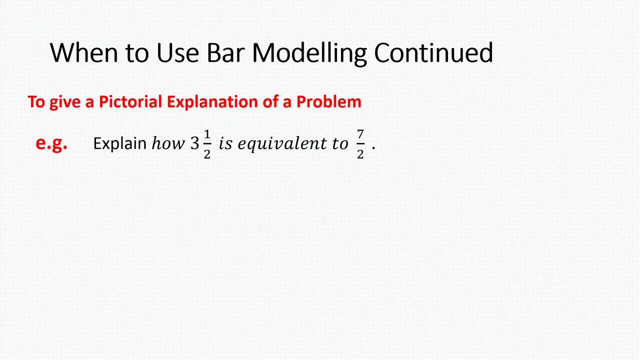 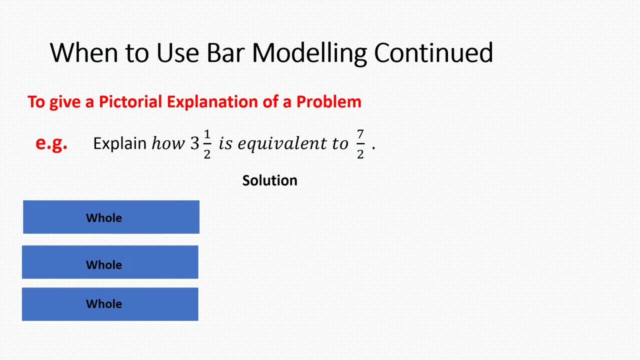 example. suppose if you had to show how three and a half is equivalent to seven hours, the first thing i will do is to model three and a half. recall if i represented a hole with a rectangular bar. all the other holes must be of similar width and length so that we emphasize. 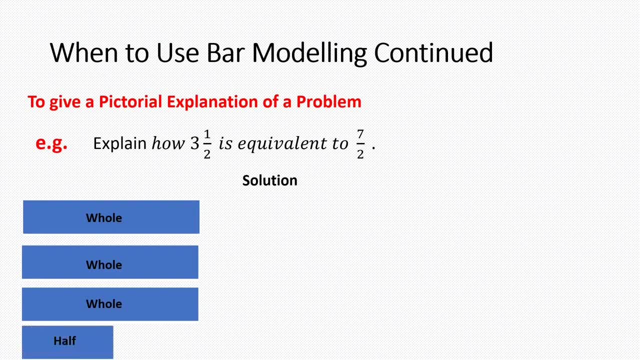 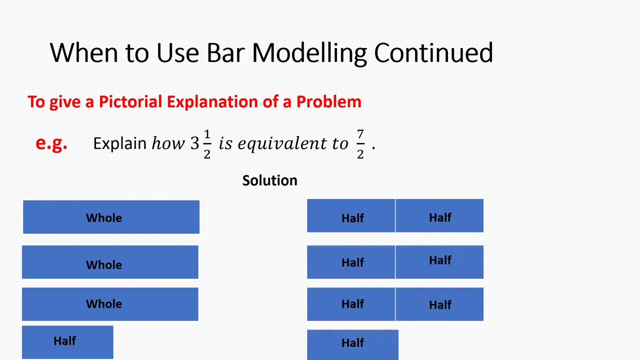 here again, spatial equality. a half, therefore, would be one of this rule, cut into two equal parts, so this represents three and a half. the whole divided into two equal parts. each part will be a half, and so therefore, the other hole would have two halves and the other hole to have the half remain as a half. 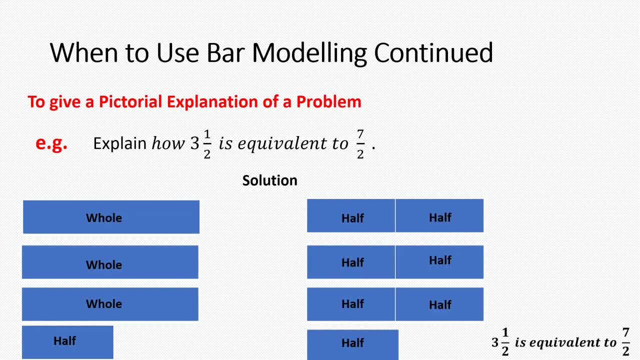 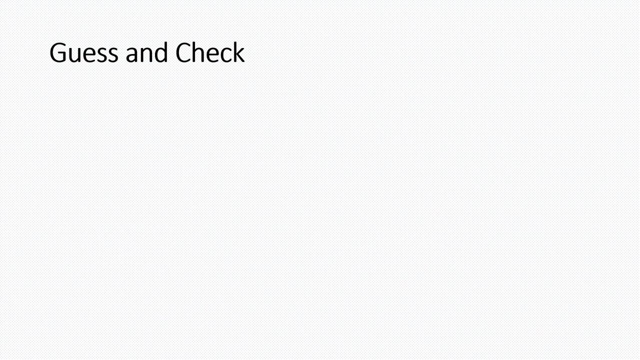 now visually you can see that three and a half is equivalent to seven halves. you can actually count them one, two, three, four, five, six, seven. the second of the three problem solving strategies we will use is guess and check. suppose you were given this example. three times a number plus five is equal to twelve and a half from your number. 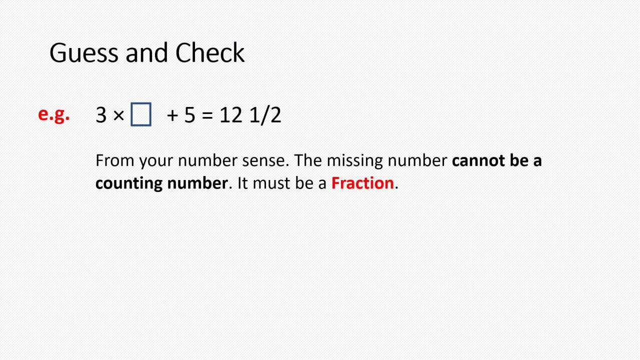 sense, the missing number cannot be a counted number, it must be a fraction. this would be determined because we understand how counting numbers and how fractions operate. however, for simplicity reasons, we will guess and check using counting numbers as of gauge. so my first guess is the number one. if i assume that the box represents one, then i can check to see if my 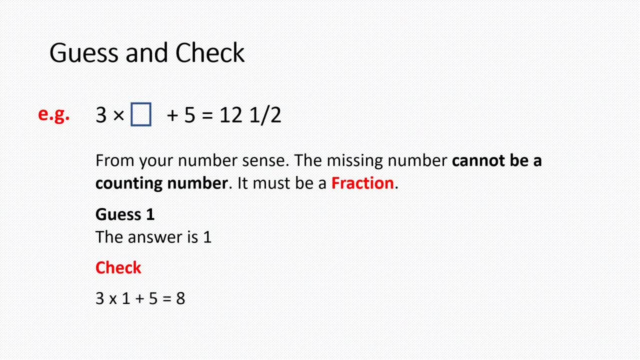 answer is correct. three times one plus five will give me eight. this clearly does not match with our answer, so my next guess would be the answer is two. now i can check to see if my answer is correct. so my third guess will be the answer is three. now let me check. when i check by substituting: 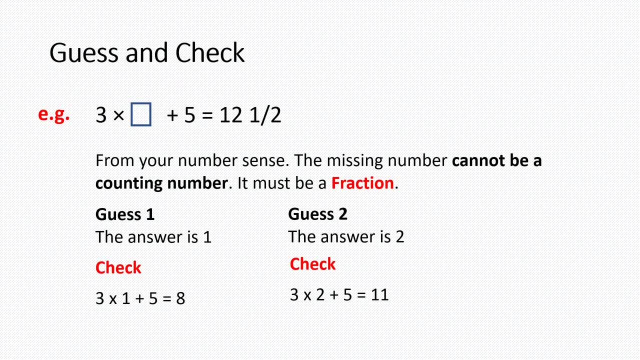 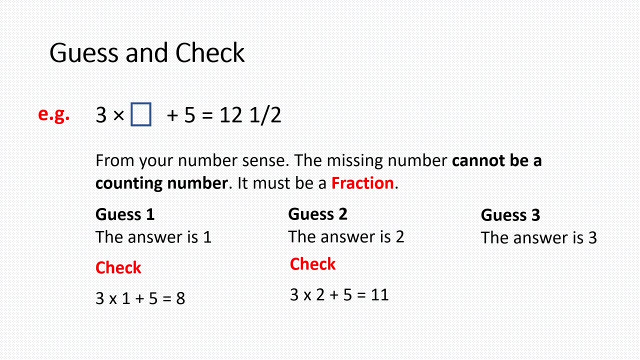 two in the missing box. so i will now have three times two plus five. recall the order of operation here? three times two is six and six plus five is eleven. this clearly does not give me the answer, so i will move on to the next number closest to two. so my third guess will be: the answer is three. 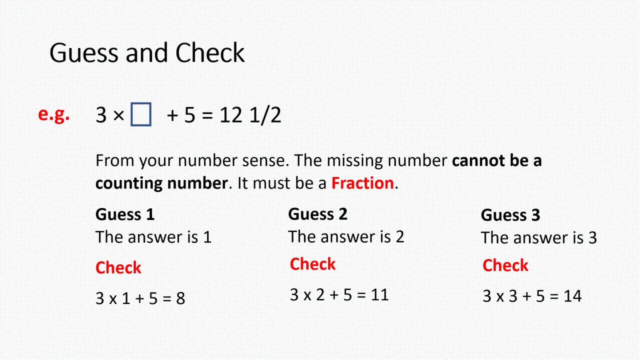 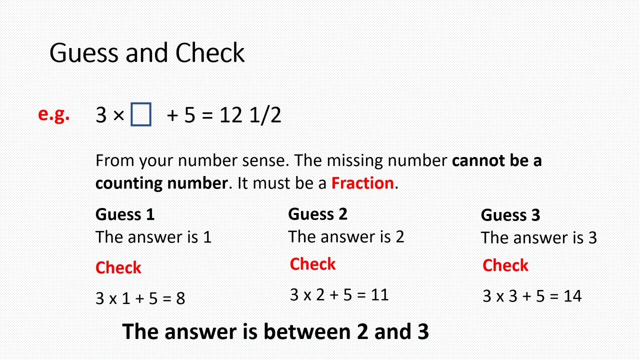 so i will have three times three plus five, but three times three is nine, and nine plus five is fourteen. clearly, this is not the answer. however, what this does is give me an idea where the answer lies, and the answer lies between two and three. this is what i know for sure. the answer is between: 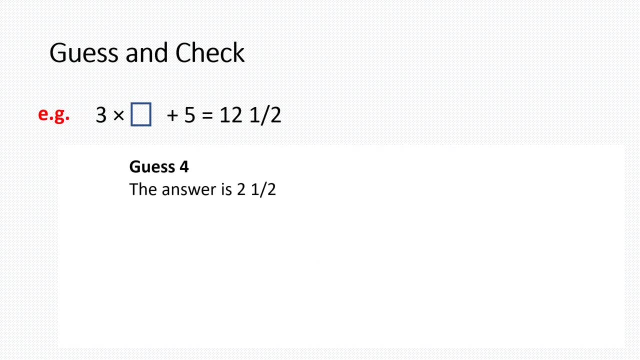 two and three. so i'm going to guess one more time. my fourth guess would be the answer is two and a half, because two and a half is somewhere between two and three. so now i'm going to substitute two and a half in the box. so i will check. 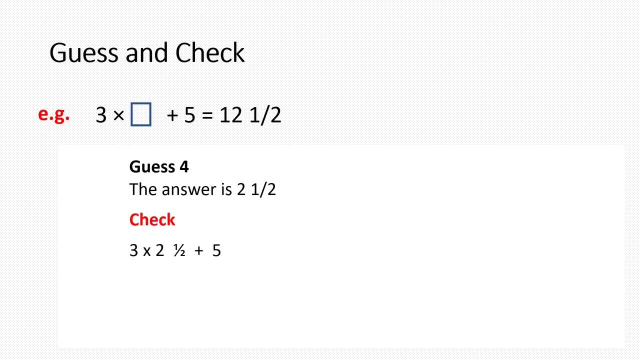 three times two and a half plus five. remember, we are going to change this mixed number to an improper fraction, so we are going to have three times five over two plus five. this will give me two plus five. but remember fifteen over two is the same as saying seven and a half and the seven and 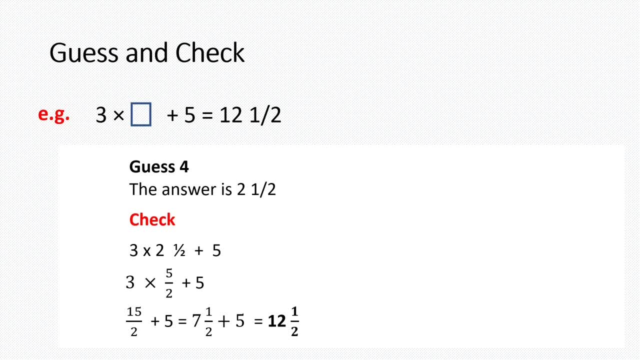 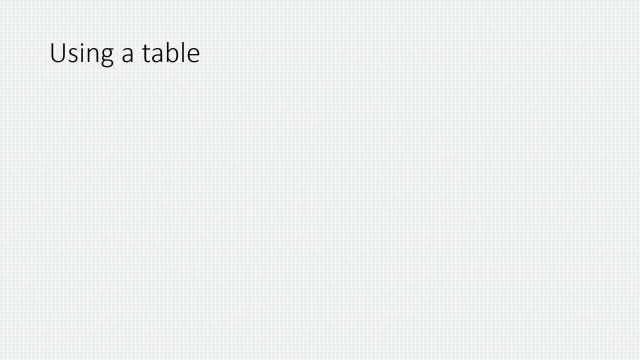 a half plus five would give me twelve and a half. this is the answer i was looking for. this therefore tells me that the missing box represents two and a half. two and a half, therefore, is your answer. the third problem-solving strategy is: the problem-solving strategy we will be looking at is using a table. this table is particularly useful for the decimal fraction. 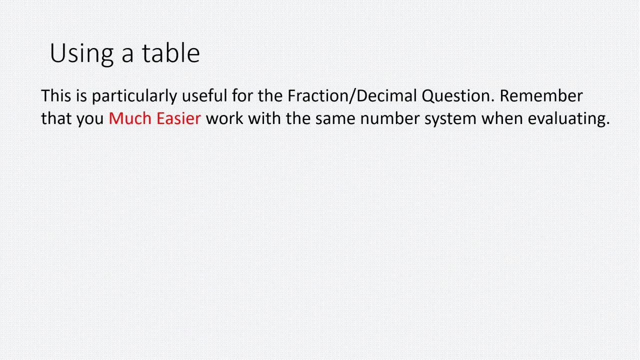 question in the third section. remember it is much easier to work with one number system when you are evaluating the problem. that is to say, if you are working with fraction, work with fractions. if you are working with decimals, work with decimals. if you are working with percentage, work with percentage. here's an example. i might spend a third of his system. 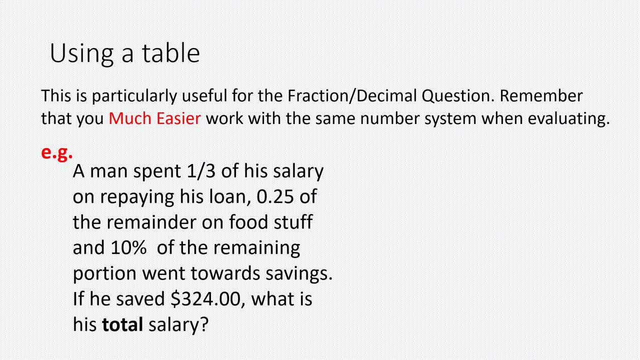 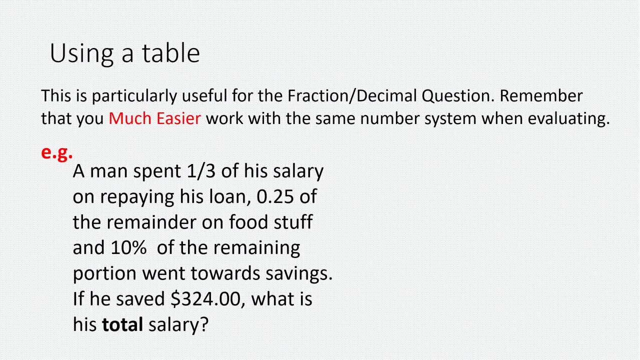 salary on repaying zero, 0.25 of the remainder on the stop and 10 of the remaining portion went towards saving. if he saved 340 dollars, what is his total salary here? let's draw our table. in our table i will put the portion of the salary that is. 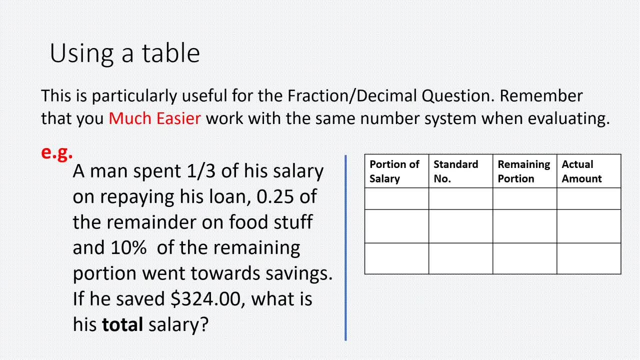 whether it was given in fraction, decimal or percentage standard number, and that is where we are going to standardize the number system in which we are representing. the remaining portion would be that amount remaining after the activity, that is, after spending on salary or spending on food or savings, and the actual amount. 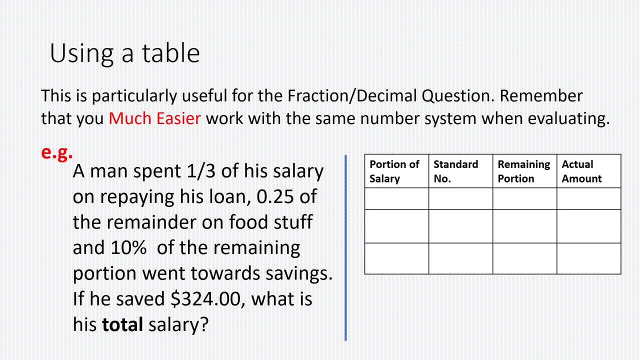 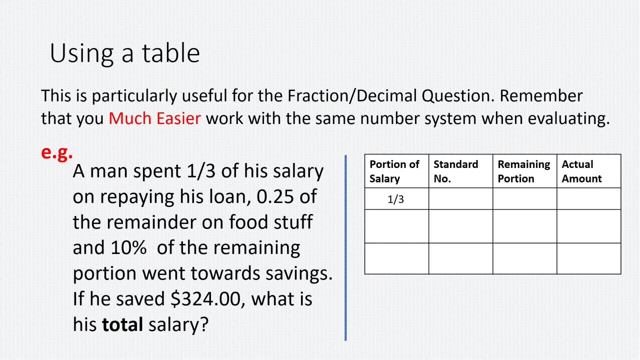 would be the corresponding amount in dollars for the portion that was described. now we had a third of his salary going towards you. if we chose to standardize all the number system using fraction, then the standard number would be a third. the remaining portion, therefore, will be two-thirds. 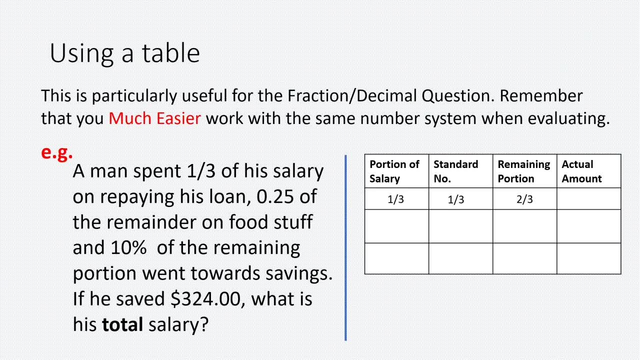 we got two-thirds. by subtracting one-third from the whole, that is, three-thirds minus one-third, will give me two-thirds. the second information that was given is 0.25 of the remaining amount. the remaining amount was two-thirds, so therefore we are speaking of 0.25. 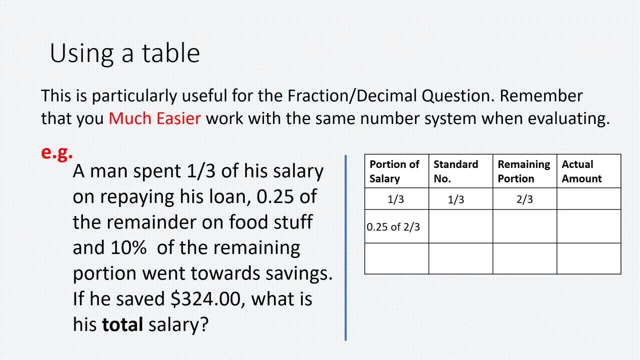 of two-thirds. but with what we are saying, we are going to be working in one number system. so we transform 0.25 to fraction, and 0.25 as a fraction would be a quarter. so a quarter of two-thirds, therefore, would be a quarter multiplied by two-thirds. 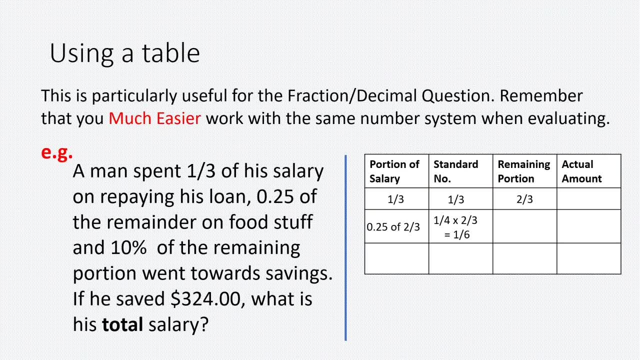 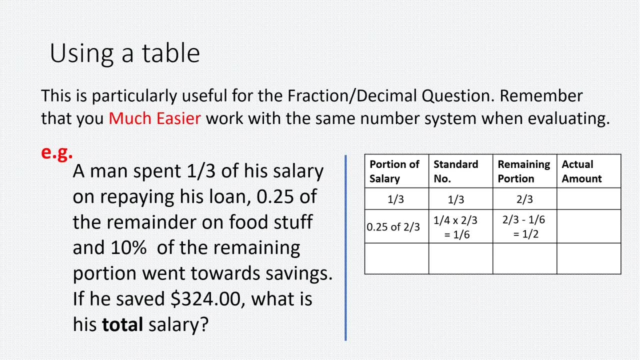 and this will give me one-sixth. the remaining portion now would be two-thirds minus one-sixth. this would give me a half. now, the final bit of information they gave us is that ten percent of the remaining portion went towards saving. so ten percent of the remaining portion, which is a half, is represented as this: 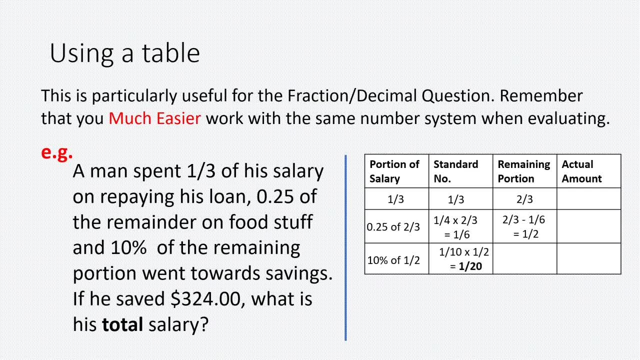 however, when standardized ten percent is one over ten, one over ten multiplied by a half now is equivalent to one over twenty. this means that one twenty-eight of his entire salary was spent on saving and recall, the actual amount that was saved is 324.. now we can get into the term前icic. 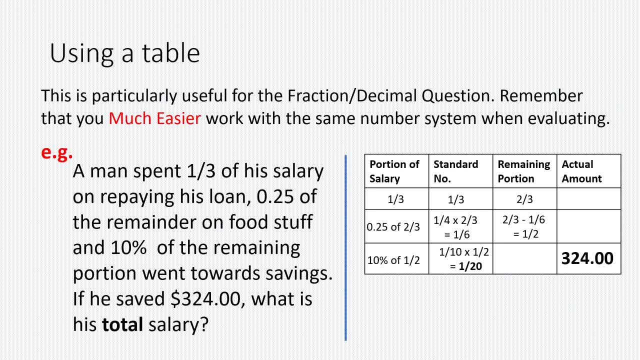 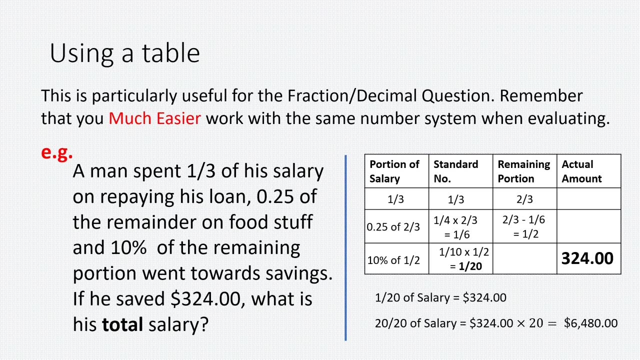 and we call: the actual amount that we see is 324.. Now we can get into calculation We had: 1, 20th of the salary is equivalent to $324.. So 20- 20th of the salary would be equal to $324 times 20, which is equivalent to $6,480.